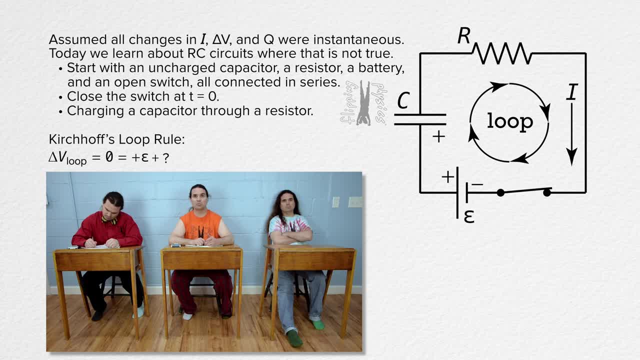 On the bottom plate of the capacitor. negative charges will be pushed opposite the direction of the current and will build up on the top plate of the capacitor. That means the electric potential will go down as we go across the plates of the capacitor in the direction of the loop. 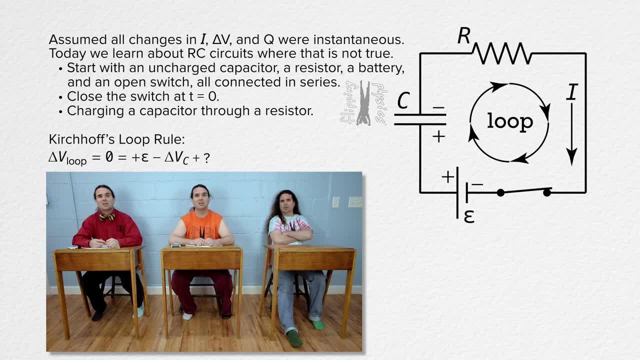 So we subtract the electric potential difference across the capacitor. I thought negative charge carriers or electrons were really the only thing which moved to cause current in electric circuits. Sure, that is what is really happening. However, we always work with conventional current, which is the direction positive charges. 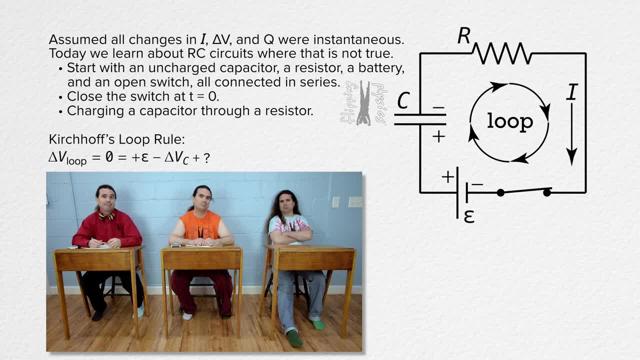 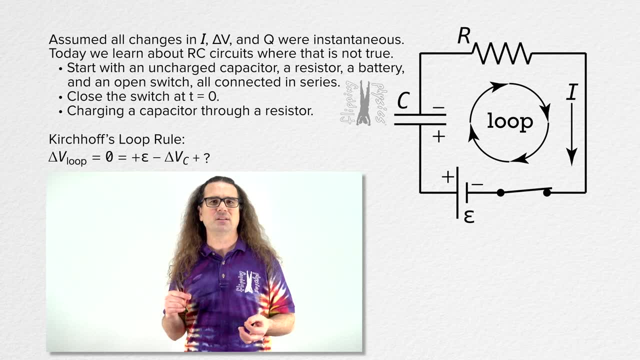 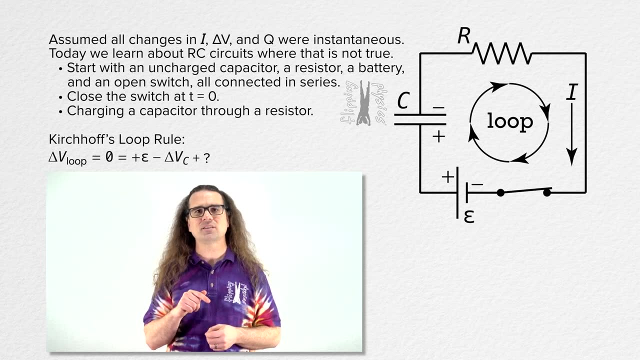 would flow if they were actually moving. So do positive charges actually build up on the bottom plate of the capacitor? Actually, positive charges do not build up on the bottom plate of the capacitor. What actually happens is that electrons are moved off the bottom plate, which causes a net positive charge. 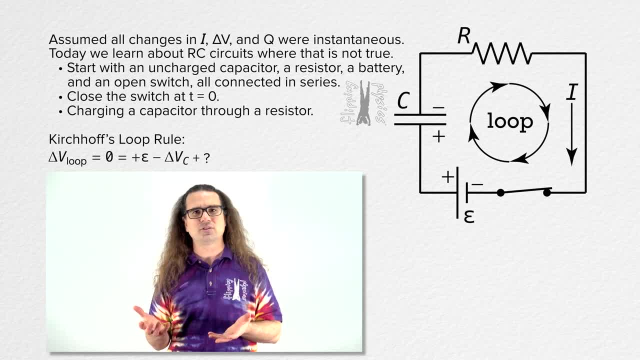 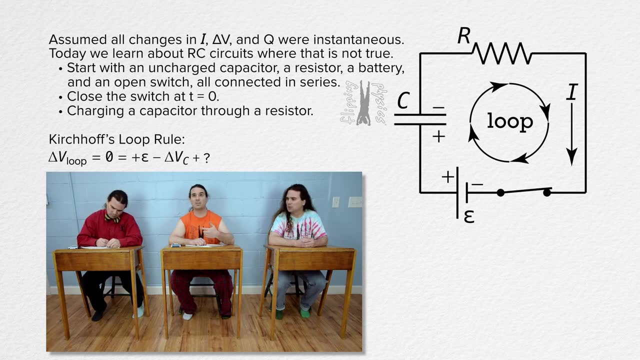 on the bottom plate. However, this is a good general representation of what occurs and helps the circuits. So let's keep Bobby's approximation of what is going on here. Bobby, Okay, next is the resistor. In a previous lesson we determined that electric potential goes down. 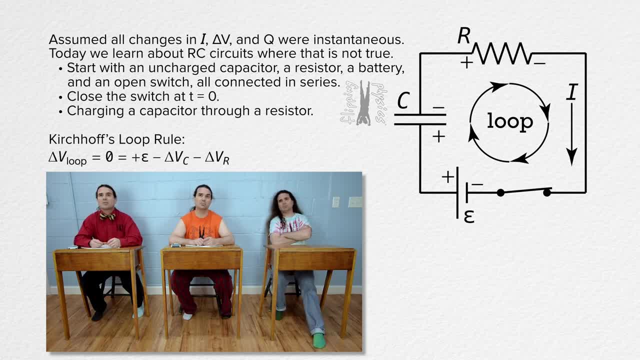 when moving in the direction of the current across a resistor. So we subtract the electric potential difference across the resistor Bo. please substitute equations in for electric potential difference across the capacitor and the resistor. Sure, We know capacitance equals charge over electric potential difference. 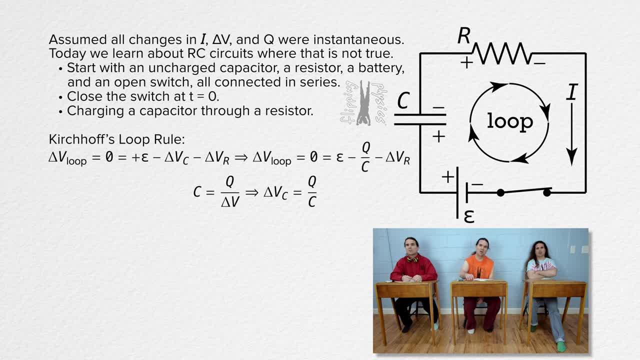 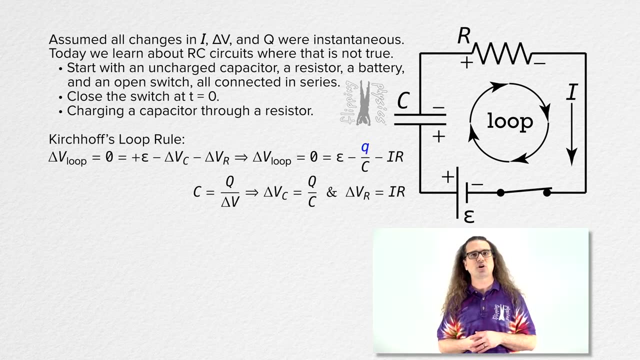 The electric potential difference across the capacitor equals charge over capacitance. We know Ohm's law states that the electric potential difference across a resistor equals the current through a resistor times the resistance of the resistor. Thank you, Bo. However, we are going to use a lowercase q for charge because the charge is. 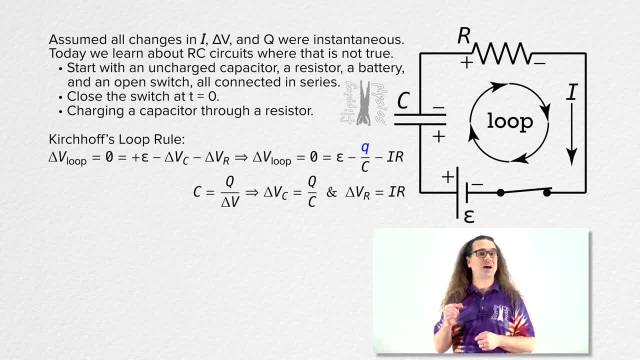 changing as a function of time And we are going to use lowercase i for current because the current is also changing as a function of time. So please realize, charge q and current i are both changing as functions of time in this Kirchhoff's Loop Rule equation. 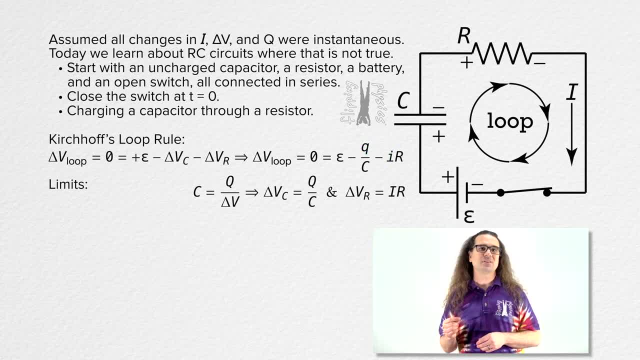 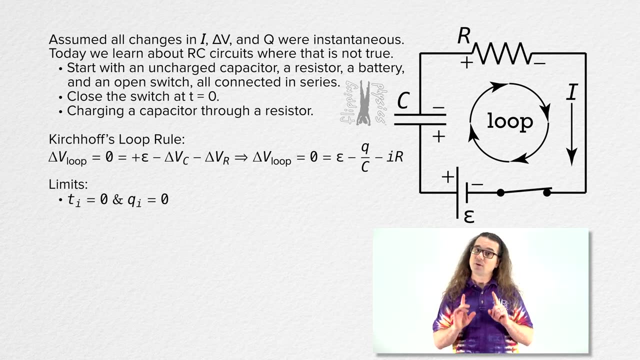 Okay, let's look at limits, Starting with time. initial equals zero. we stated earlier that we are charging a capacitor through a resistor and that the capacitor starts with zero charge on it. Therefore, the initial charge on the capacitor equals zero. Realize: 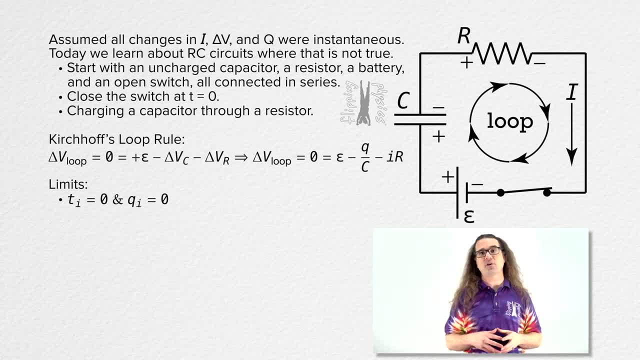 that also means the initial electric potential difference across the capacitor is also zero. You see, that is true from the equation싲 for electric potential difference across the capacitor which Bo gave us. Billy, please use the Loop equation to determine the initial current in the circuit, Absolutely From the Kirchhoff's Loop Rule. 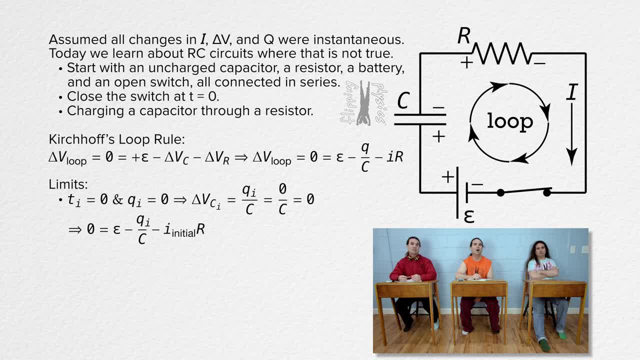 equation we know: zero equals the EMF across the battery minus. Well, the initial charge is zero. so zero divided by the capacitance of the capacitor minus …. Well, the initial current in the circuit times the resistance of the resistor. That means initial current times. resistance equals emf. 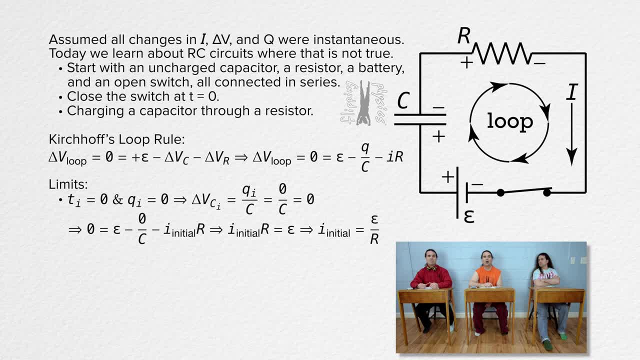 So the initial current in the circuit equals the emf across the battery divided by the resistance of the resistor, Oh. and because the charge of the capacitor will increase as a function of time, electric potential difference across the capacitor will also increase over time. 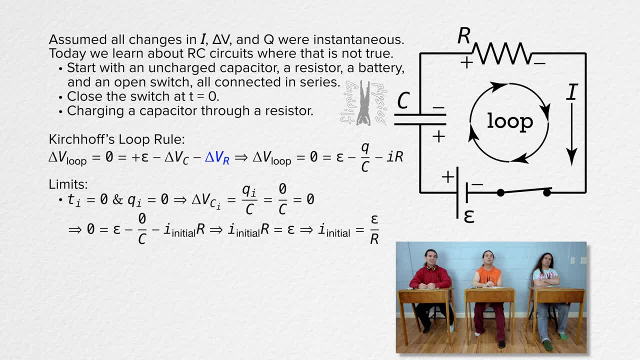 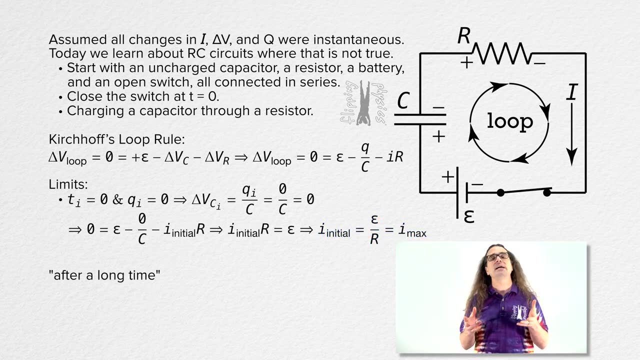 This means the electric potential difference across the resistor will decrease over time And that means the current in the circuit will decrease as a function of time. In other words, the initial current in the circuit is also the maximum current. Thank you, Billy. Now let's look at the limit. after a long time, Please realize. 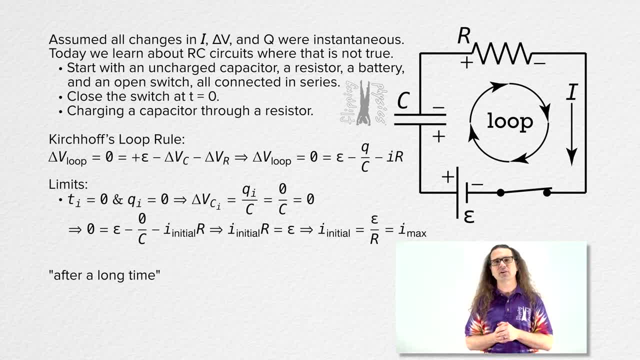 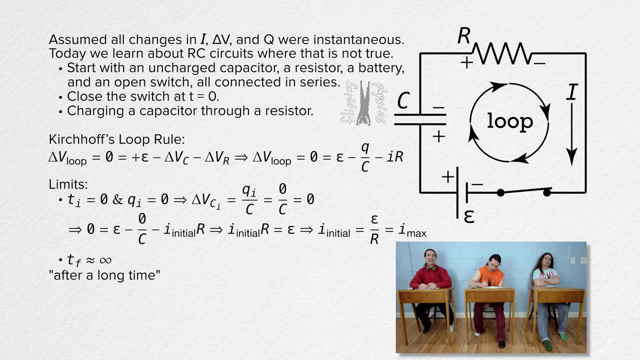 after a long time in the parlance of RC circuits means you can consider time final to be equal to approximately infinity. Bo tell me what you know about this RC circuit after a long time, or roughly an inch. Well, the current starts at its maximum value and decreases the entire time. So 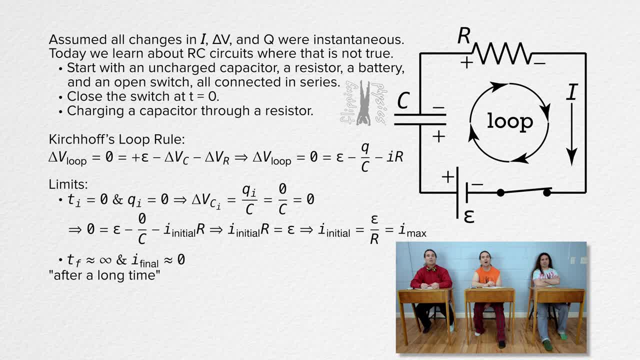 after a long time the final current in the circuit is roughly zero. That means the electric potential difference across the resistor also equals zero. You can see that from Ohm's law. Substituting current final of zero into the loop equation shows us: 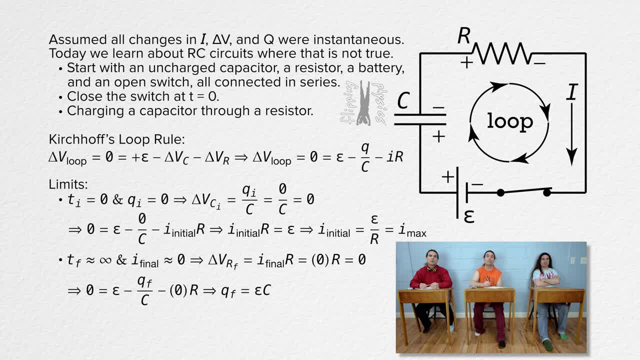 that the charge final on the capacitor equals the emf across the battery times, the capacitance of the capacitor. And because we know the charge has been increasing this whole time, we know the charge final on the capacitor is also the maximum charge on the capacitor. 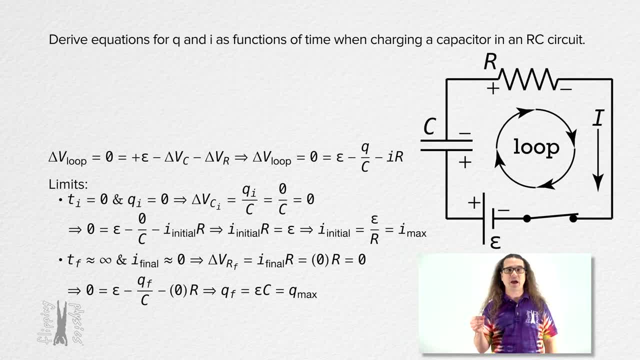 Well done, Bo Thanks. Now we are about to derive equations for charge and current as functions of time. However, before we do, I want to point out that AP Physics C, electricity and magnetism students are responsible for knowing how to derive these equations. 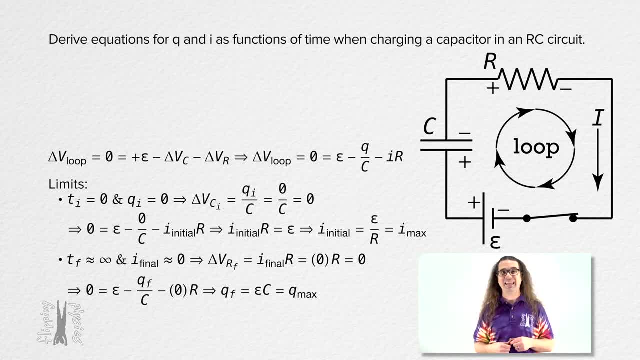 So, yes, you need to understand these derivations and you need to be able to do them on your own. And actually we already did a derivation very similar to this when we derived the equations of motion with a drag force, if you remember that from AP Physics, C Mechanics- 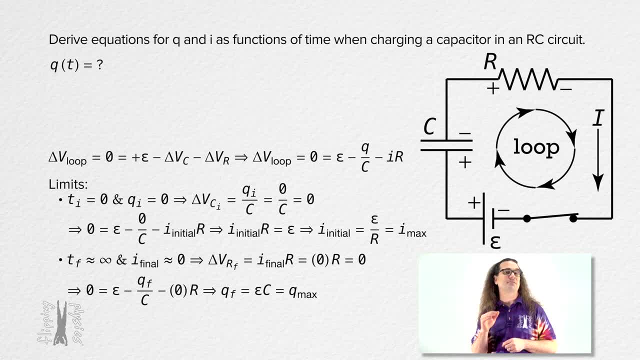 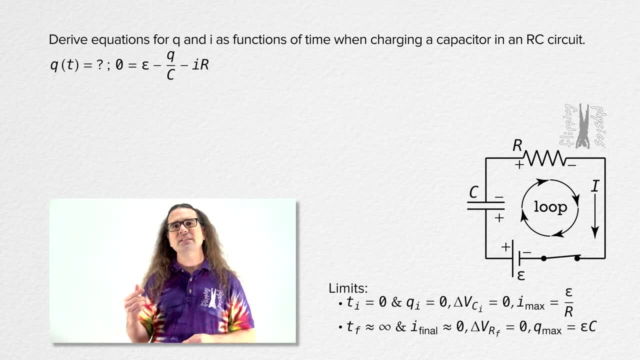 Okay, let's start by solving for the charge on the capacitor as a function of time. Here we go, Starting with our Kirchhoff's loop rule equation. we move current times, resistance to a to the other side of the equation. Divide the whole equation by resistance. 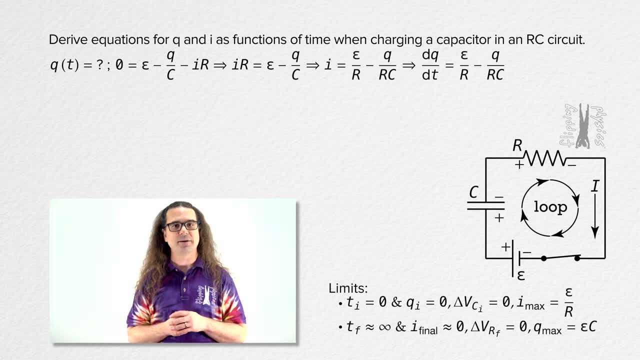 We know current equals the derivative of charge with respect to time, And actually let's pause here for a moment. Typically on an AP Free Response question where they ask you to solve for something like this, they will actually put it in two parts. 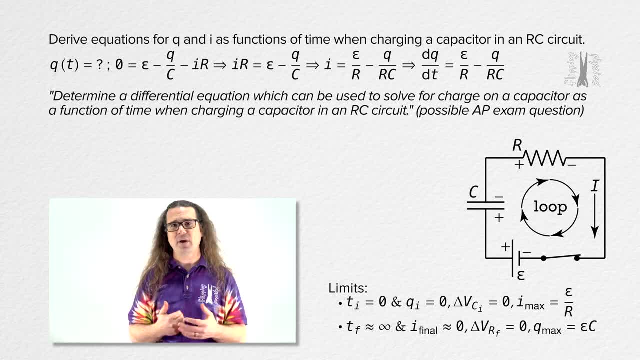 First, they ask you to determine a differential equation which can be used to solve for whatever you're solving for. In this case, charge on the capacitor is the derivative of charge. So, on the capacitor as a function of time, This equation right here, the derivative of charge. 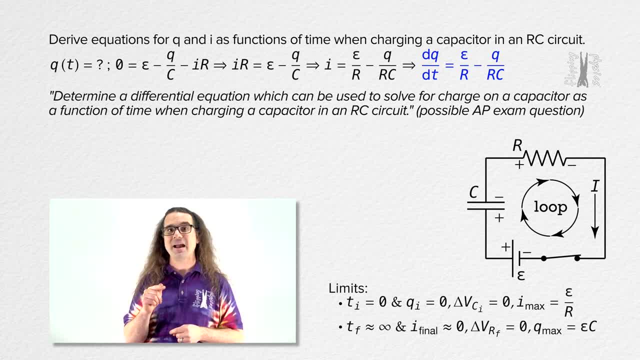 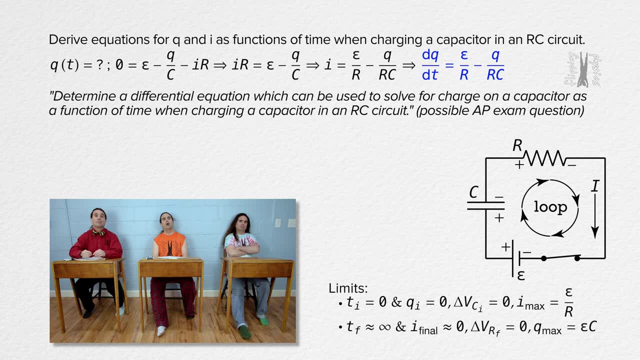 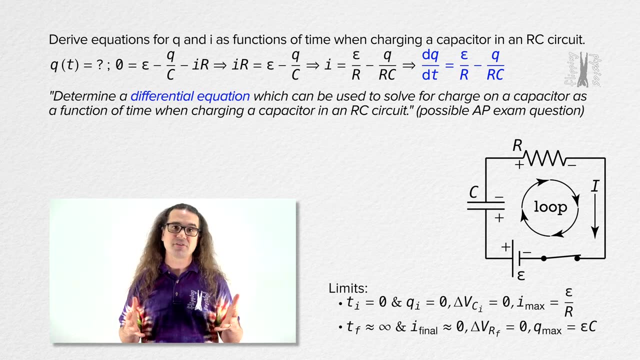 with respect to time, equals electromotive force over resistance minus the charge over the quantity resistance times. capacitance is the answer to that question. This equation is the differential equation which can be used to solve for charge on the capacitor as a function of time. I figured it. 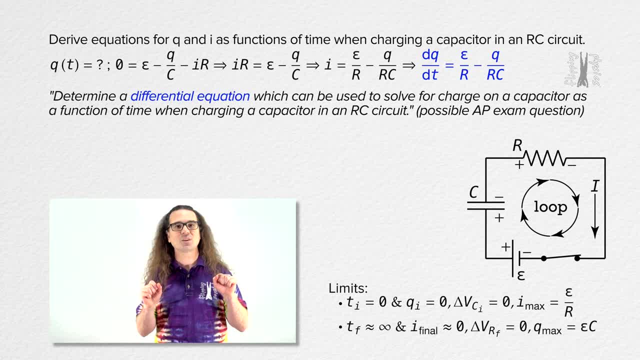 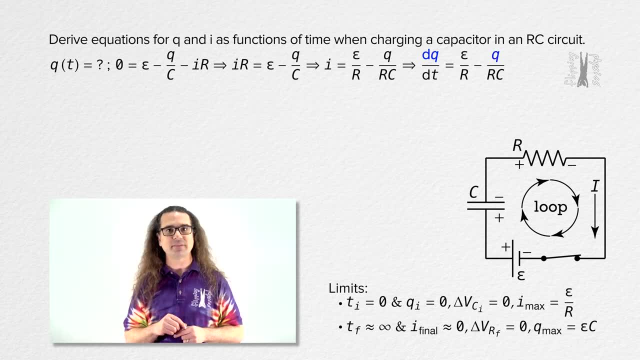 would be helpful to know that It is: Thanks, Yeah, thanks, Okay, back to the solution. Our goal here is to: Okay, back to the solution. Our goal here is to to get dq and q on the left-hand side of the equation and dt on the right-hand side of the. 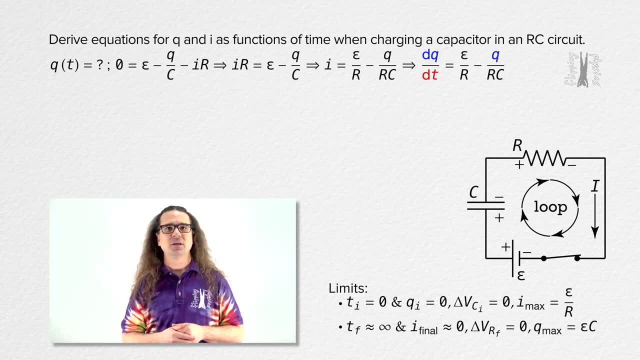 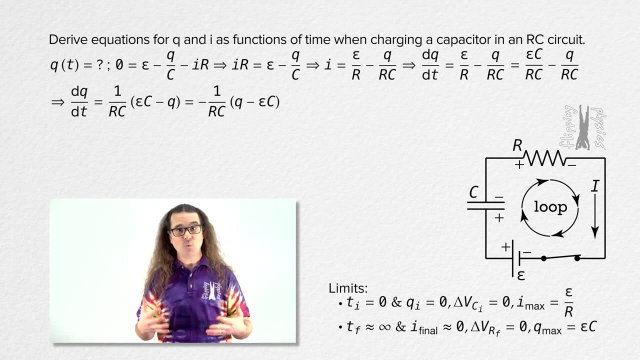 equation so we can take the integral of the whole equation. To do that, we start by getting a common denominator of resistance times capacitance. on the right-hand side We can factor out the inverse of resistance times- capacitance and then factor out a negative one from the parenthetical expression. 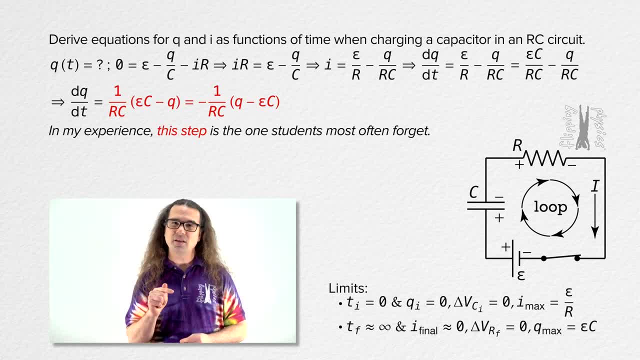 on the right-hand side. I do want to point out that this particular step where we factor out negative one is the one step I find students most often forget. so please remember to factor out negative one at this point in the derivation. I'll make a special note of that, Mr P. 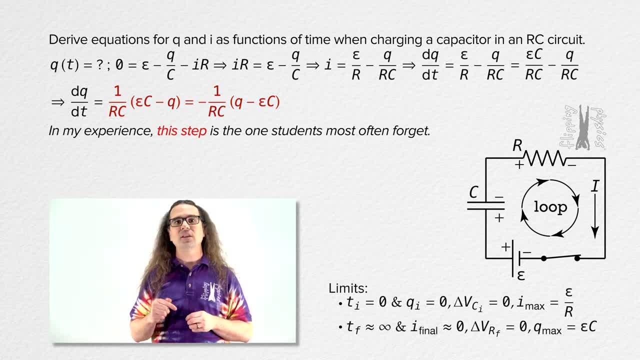 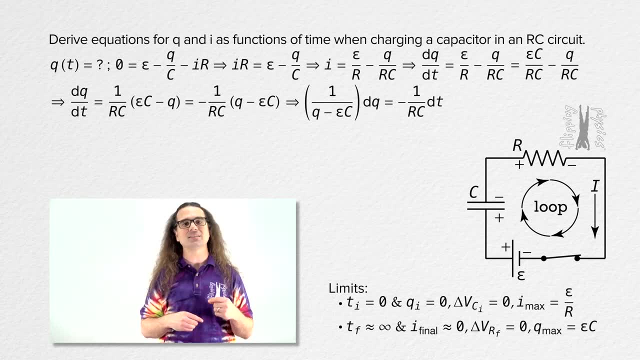 Thank you, Billy. Next, we divide the whole equation by the quantity charge minus electromotive force, times, capacitance, and we multiply the whole equation by dt, And then we take the integral of the whole equation On the left-hand side. we are at: 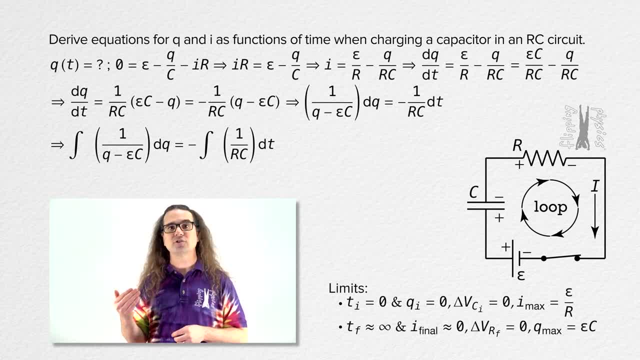 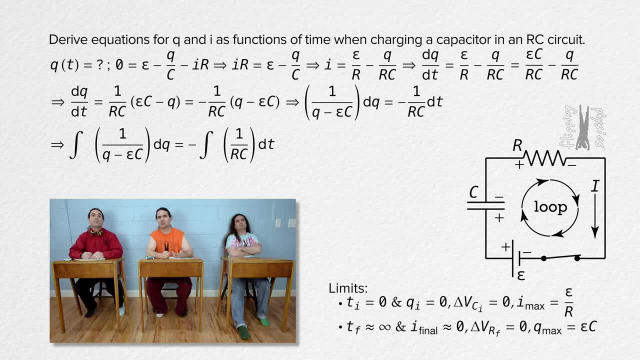 taking the integral with respect to charge. so our limits are in terms of charge, Bobby. what are those limits? Well, the initial charge on the capacitor is zero, so the initial limit is zero. The final charge on the capacitor is charge maximum or emf times capacitance. 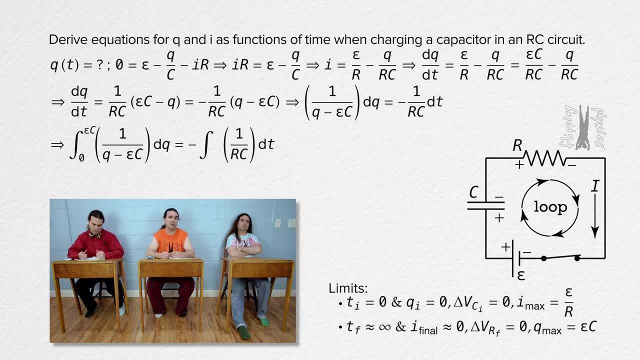 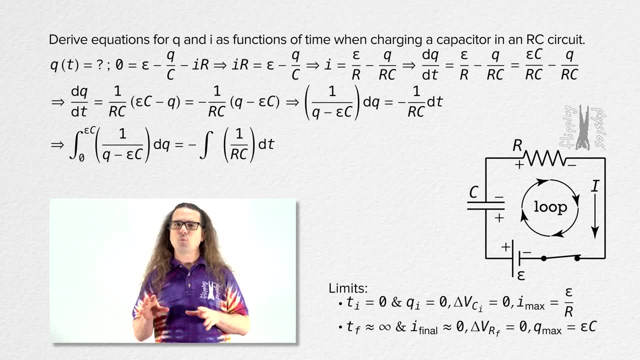 so emf times capacitance is the final limit for charge. Actually, Bobby, I know the final charge on the capacitor is the electromotive force times the capacitance. However, what we are solving for here is the charge as a function of time. So our final limit for the charge is the charge at some time t. 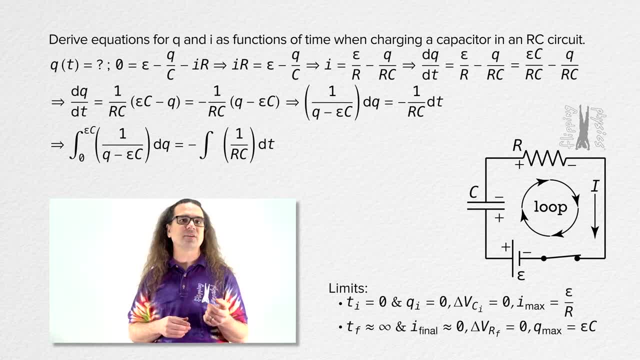 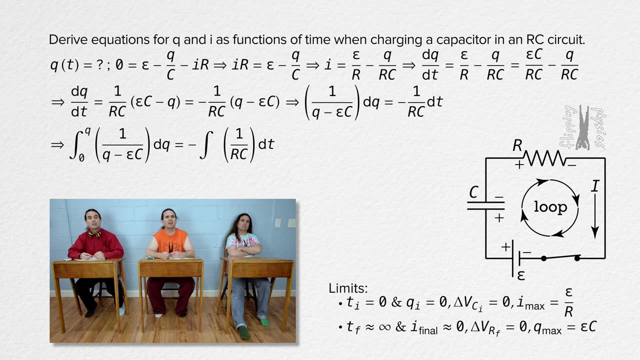 after we close the switch. In other words, the final limit on charge is the variable lowercase q, which represents the charge at time. t, Bobby, what then? do you think the integral limits are on the right-hand side? Okay, On the right-hand side, we are taking the integral with respect to time. 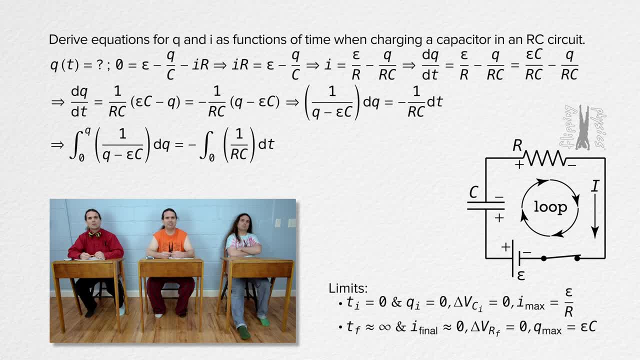 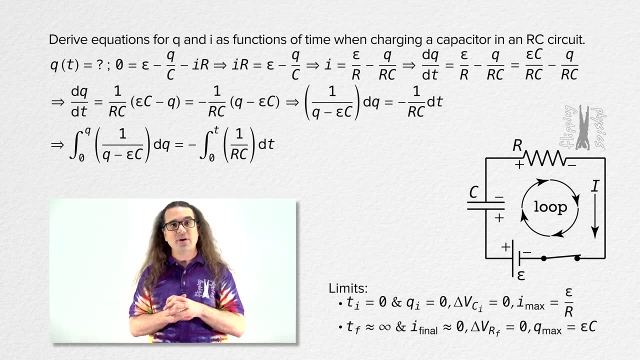 So time initial is zero and time final is just lowercase t, And that represents the time variable in the equation we are solving for charge as a function of time. Exactly, Bobby, thanks. On the right-hand side, resistance and capacitance do not change as a. 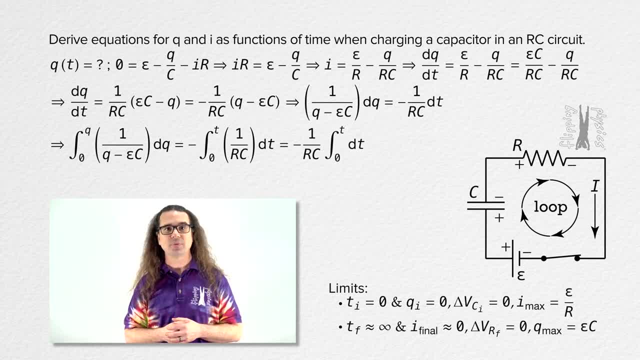 function of time. so we can take those out from the integral On the left-hand side, the integral with respect to charge of the inverse of the quantity charge minus time minus electromotive force, times capacitance is the natural log of the quantity charge minus. 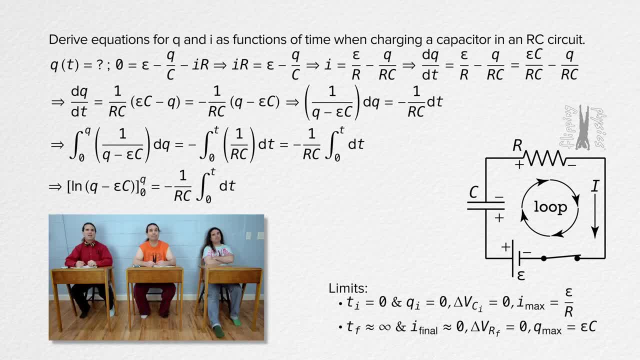 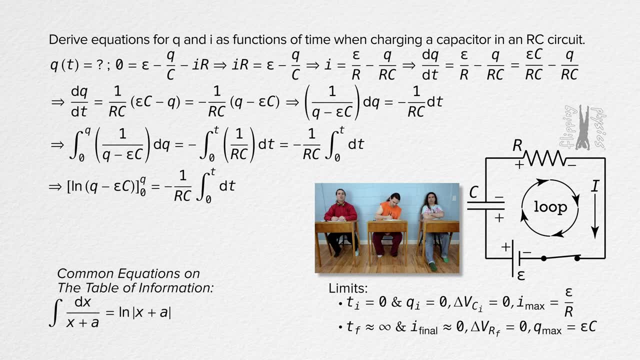 electromotive force times capacitance, What? I don't remember that. How do we know that That equation is among the common calculus equations on the table of information provided to us by the college board during the AP exam? It is. That is helpful. How did I miss that? 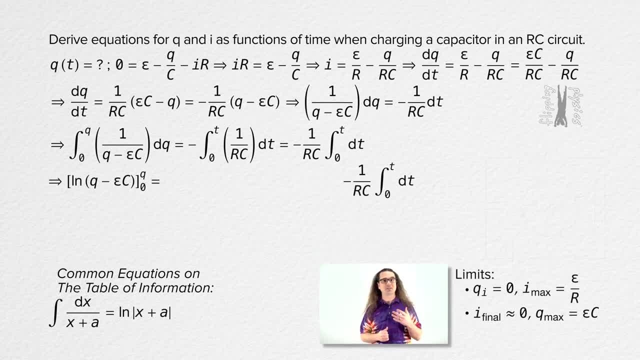 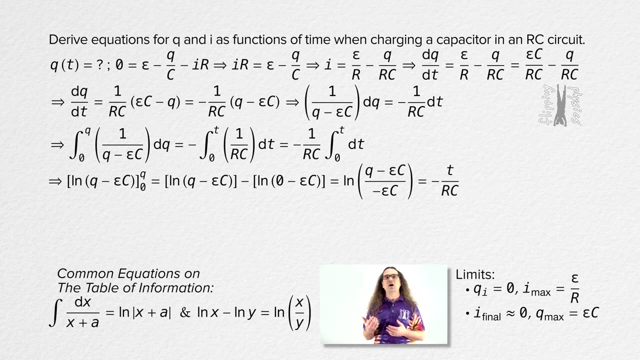 I do not know. We can substitute in the limits on the left-hand side, And the natural log of x minus the natural log of y equals the natural log of the quantity x divided by y And the integral of dt. from time zero to time, t is just t. So on the right-hand, 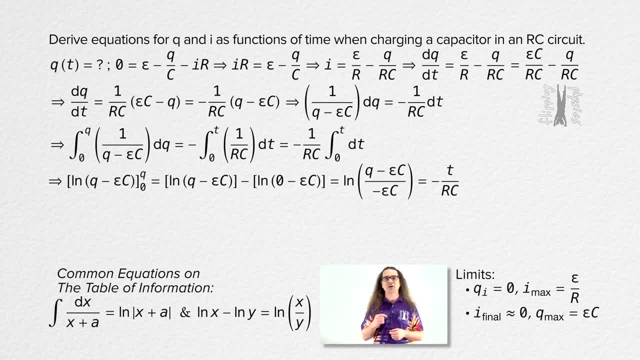 side we have the negative of time, t divided by the quantity, resistance, times, capacitance, And now we can take e to the power of the whole equation. On the left-hand side, we know e to the power of the natural log of x equals x. 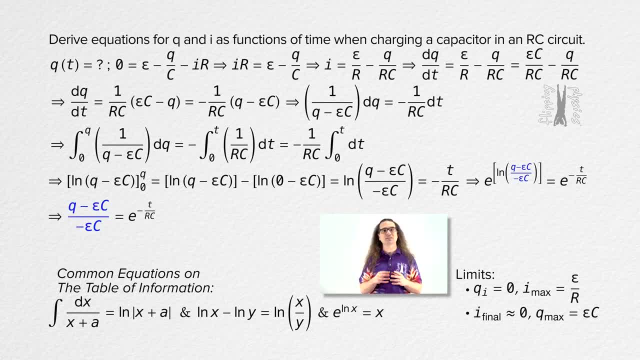 So on the left-hand side we now have charge minus electromotive force times capacitance, all divided by the negative of electromotive force times capacitance. On the right-hand side we have e to the power of the quantity negative time, t divided by the. 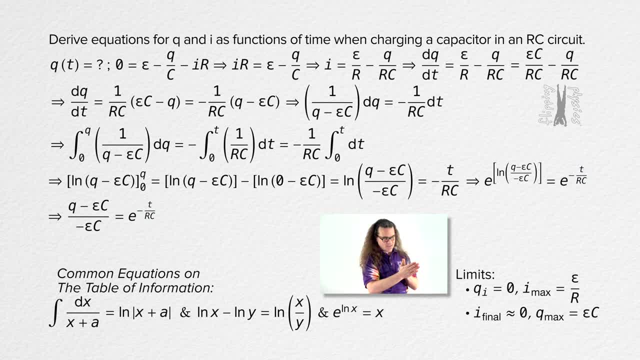 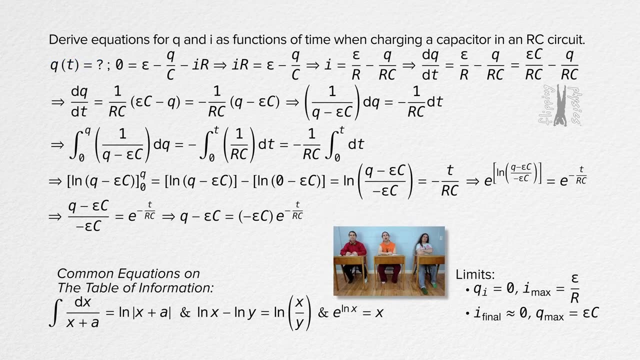 quantity resistance times capacitance. Billy, remind me what we are solving for. We are solving for the charge on the capacitor as a function of time. So we multiply through by negative electromotive force times capacitance, Move electromotive force times capacitance to the right-hand side of the equation. 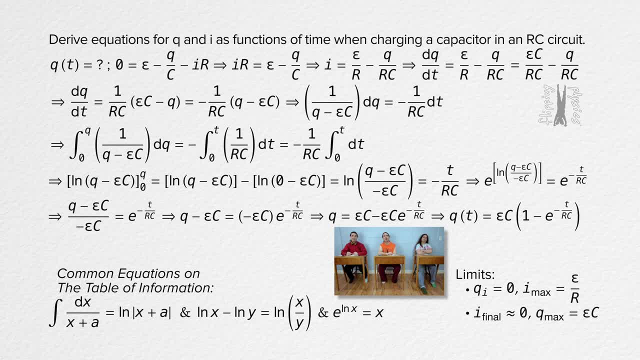 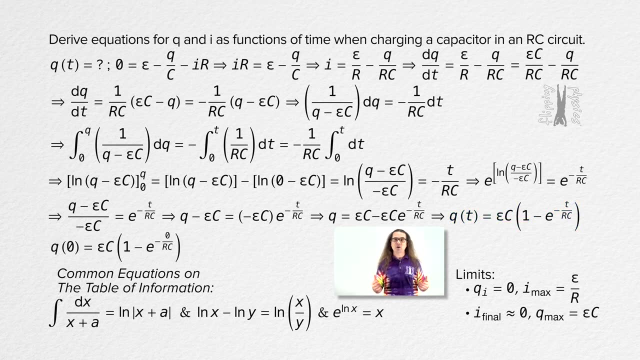 We can factor out electromotive force, times, capacitance And we have an equation for charge as a function of time when charging a capacitor in an r-c circuit. Very nice, Billy Notice. this equation fits our limits for charge When time t equals zero. 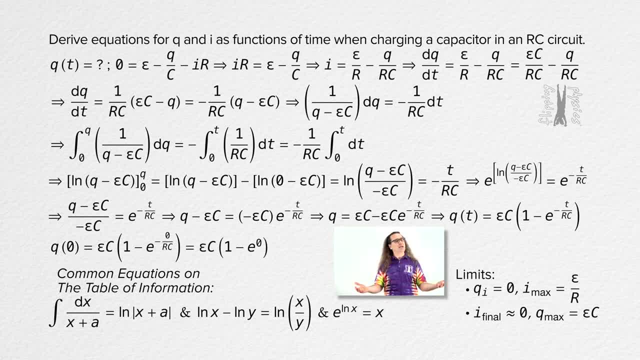 we get e to the power of this formемуands 0. Delaware Form 3: zero in the equation Class. what is the value of e to the power zero? Negative one: One Zero. E to the power zero equals one. 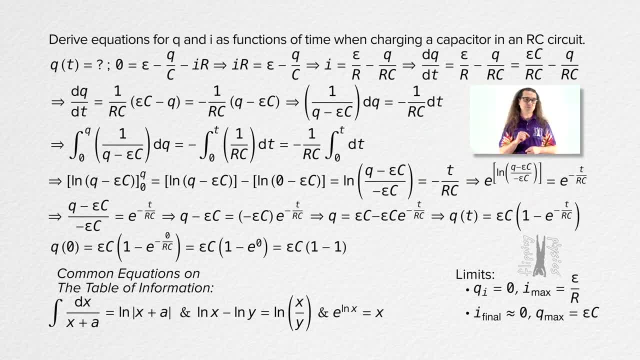 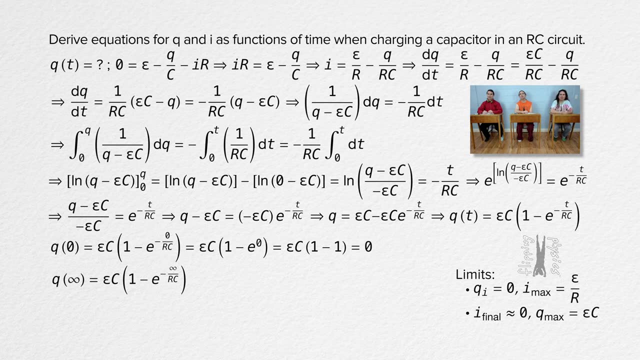 I knew that, Yes, it does. Therefore, when time equals zero, this equation shows that the charge on the capacitor is zero. Bo, what about the charge when time equals infinity? Well, if we plug infinity in for time, we get e to the negative infinity, which is zero. 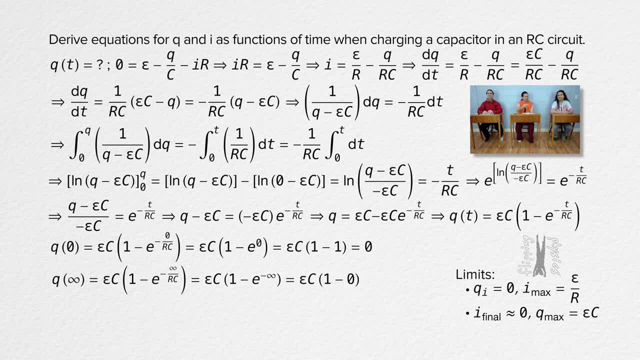 Yeah, zero, Sure, zero. I feel like you should know all of these numbers. Yeah, I probably should. So this equation shows that the charge on the capacitor after roughly an infinite amount of time equals emf times capacitance And we already showed that equals the maximum charge of the. 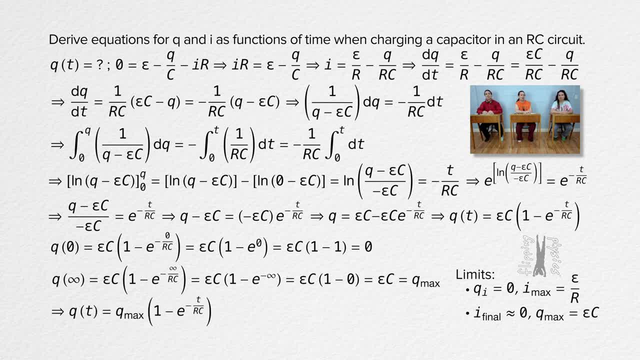 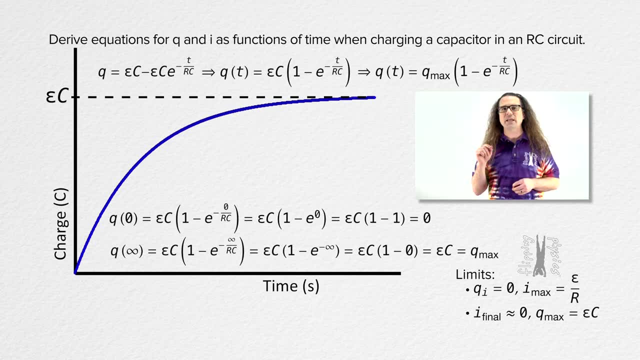 capacitor. Yeah, we could substitute charge maximum into the equation for charge as a function of time. Thanks, Bo. This is the graph for charging an initially uncharged capacitor through a resistor as a function of time. You can see. the initial charge is zero, the charge on the capacitor. 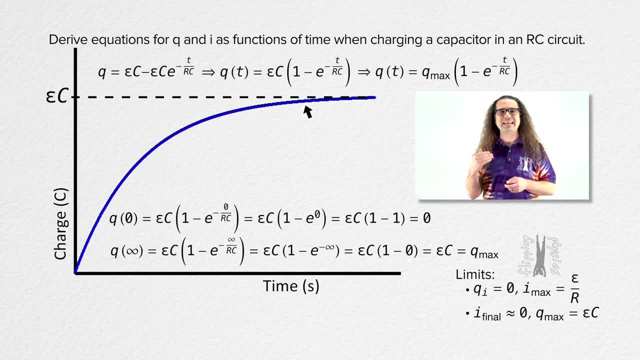 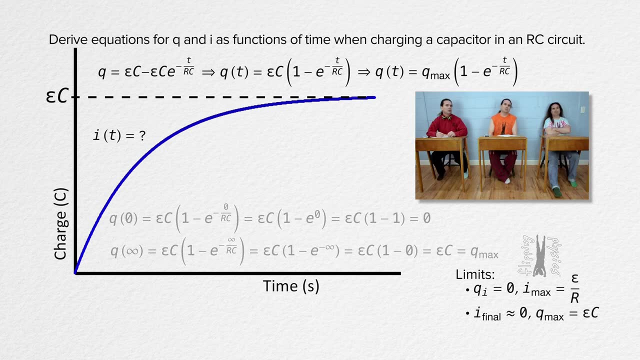 increases according to the equation we solved for, and it asymptotes to the maximum charge, which is equal to electromotive force times capacitance. Bobby, please solve for the current in the circuit as a function of time. Okay, Um, current equals the derivative of charge with respect to time. 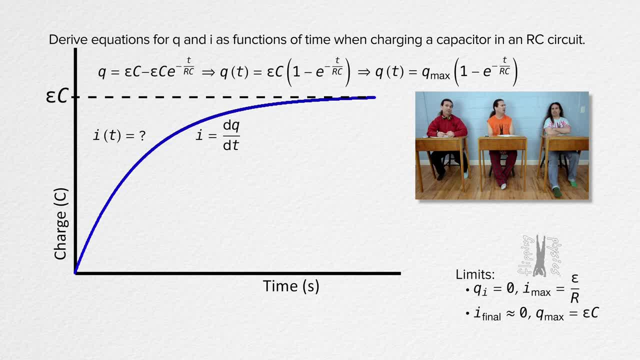 Sure, And we now have an equation for the charge on the capacitor as a function of time. Right, We can substitute the equation for charge we just solved for into that equation. Actually, could you go back a few steps and use emf times capacitance minus emf times capacitance. 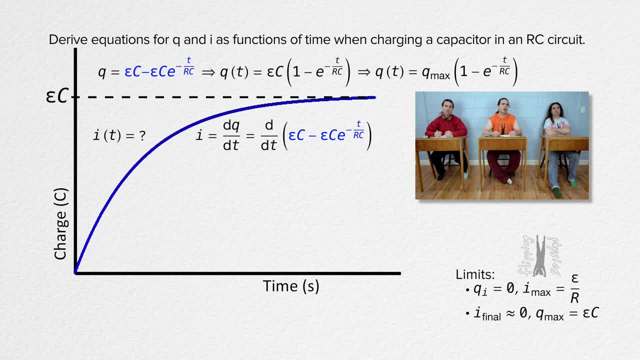 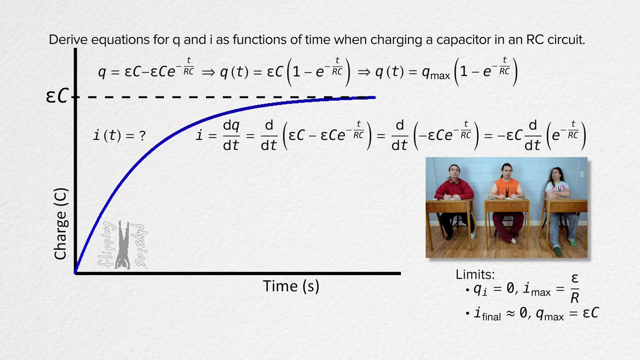 times e to the power. infinity Negative time over the quantity resistance times capacitance, Please. Okay, emf and capacitance are both constant as a function of time, So the derivative of that is zero And we can take emf times capacitance out from the derivative, The derivative of e to the 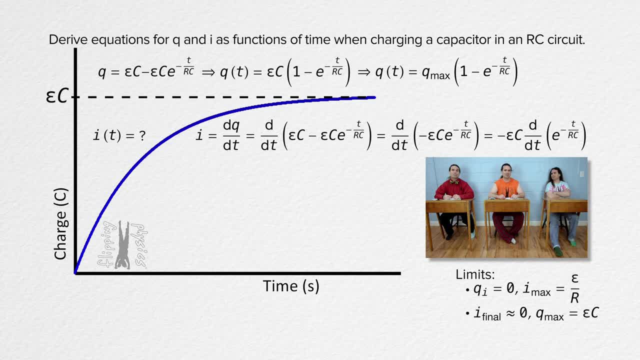 power. negative time over resistance times, capacitance. Oh, the equation for this is also on the table of information. That means the derivative of of e to the power. negative time over resistance times capacitance equals negative one over resistance times. capacitance all times. e to the power. negative time over resistance times. 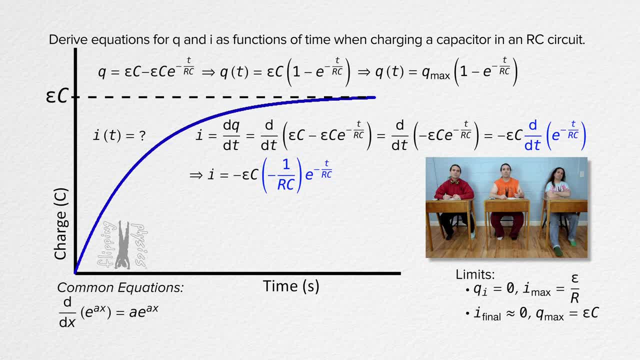 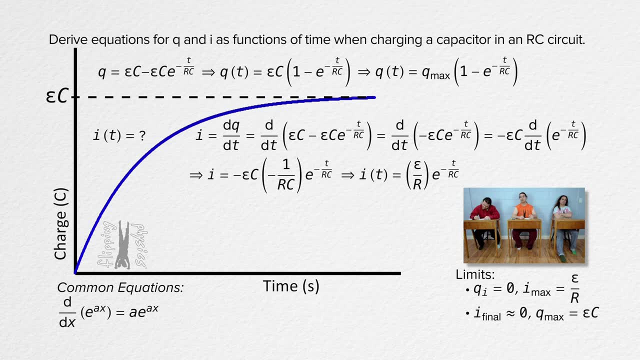 capacitance. So the current through the circuit as a function of time equals emf over resistance times, e to the power, negative time over resistance times: capacitance. Well done, Bobby. Billy, please determine the limits of the current through the RC circuit. 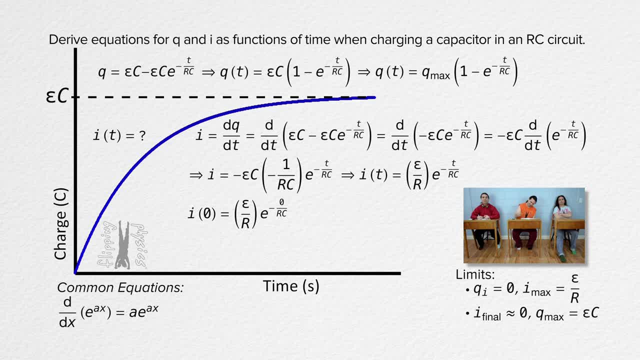 Certainly, When we substitute zero in for time, t into the equation for current, we get e to the negative zero, which equals one. So the initial current in the RC circuit equals electromotive force divided by resistance, And we already determined that is the maximum current. 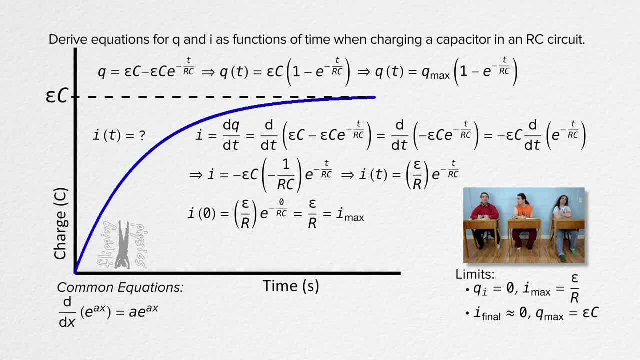 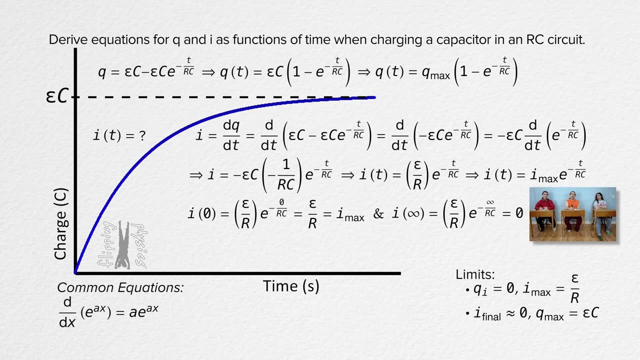 so we can substitute current maximum back into the equation for current as a function of time And for the limit after a long time. we can substitute infinity in for time. in the current equation E to the negative infinity equals zero. so the current in 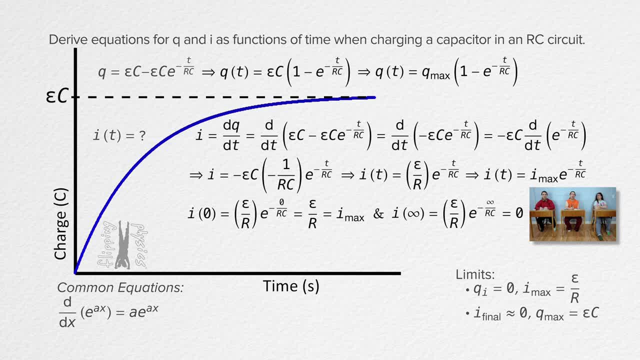 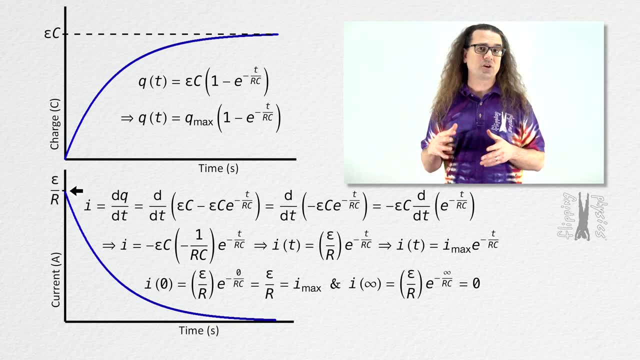 the RC circuit is zero after a long time, which is what we got before. Thank you, Billy. And this is the graph for that equation. You can see the initial current is at a maximum value of electromotive force divided by resistance, And the current decreases. 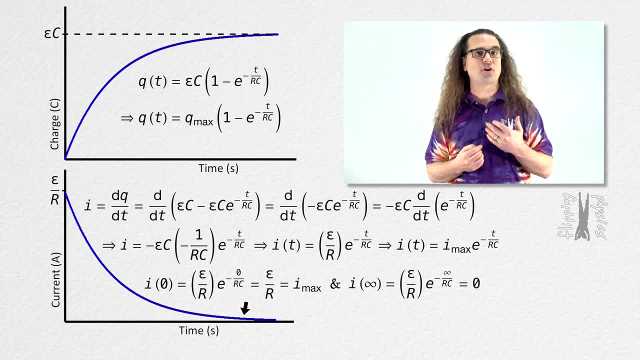 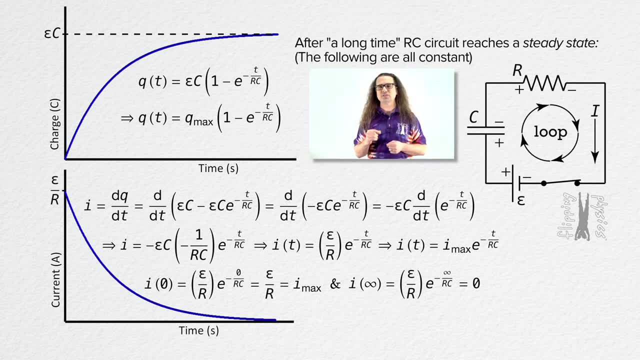 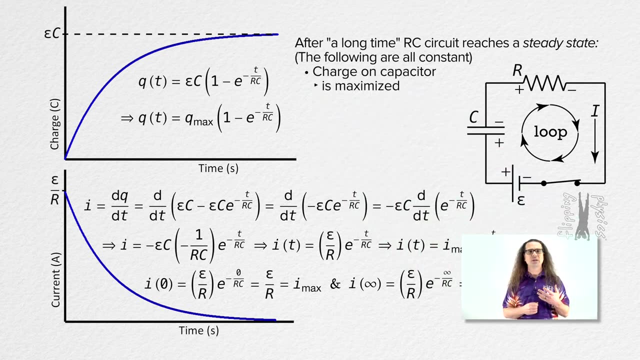 according to the equation we solved for and asymptotes at a current of zero. So notice that, according to both of our graphs, after a long time the RC circuit reaches a steady state condition where the charge across the capacitor is at its maximum value. Realize the electric. 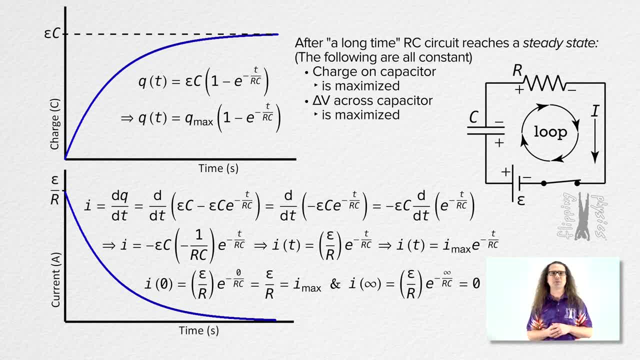 potential difference is also steady at its maximum value. We know this because the electric potential difference across the capacitor equals the charge on the capacitor divided by its capacitance. The charge has reached a steady state and the capacitance of the capacitor is constant. therefore, the electric potential difference has also reached a steady state. 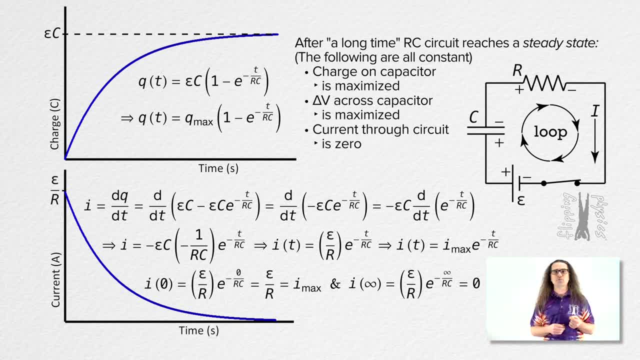 This also means that after a long time, the current through the circuit has reached a steady state value of zero And the electric potential difference across the resistor is also zero, because it equals current times. resistance and the current through the resistor has a constant value. 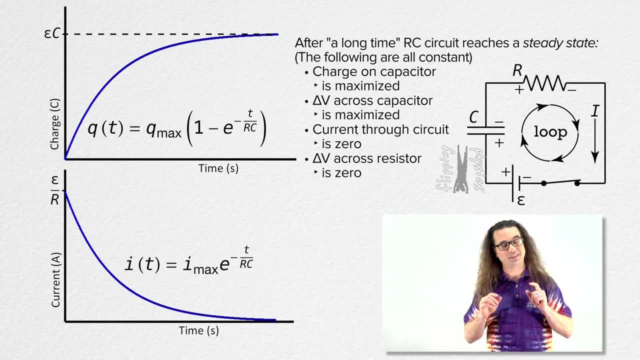 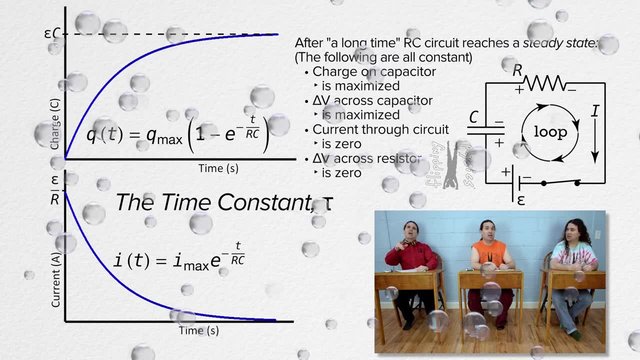 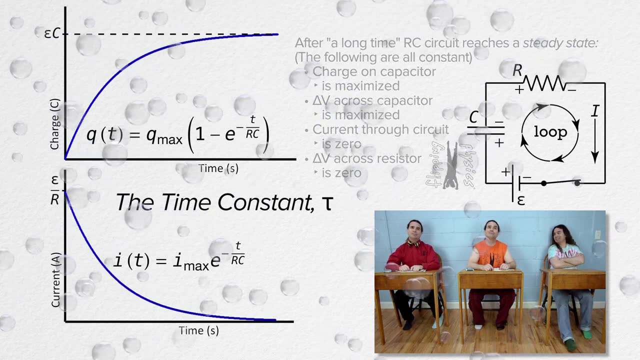 of zero. And now we get to talk about the time constant. Hey, I'm excited about the time constant. Okay, let's get on it. let's learn about the time, Both the equation for charge as a function of time and the equation for. 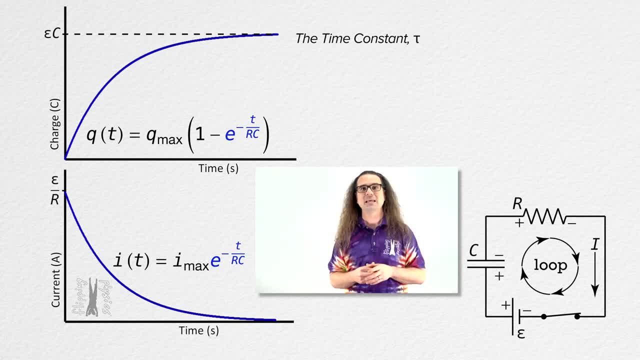 current as a function of time, have this expression in them: E to the power, negative time over the quantity. resistance times, capacitance. The time constant equals whatever variables appear in the denominator of that fraction. In other words, for an RC circuit, the time constant equals resistance times, capacitance. 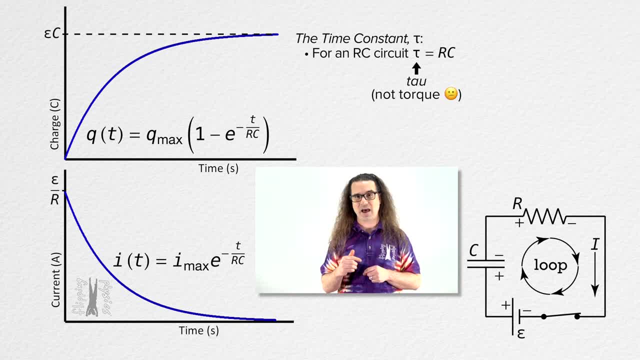 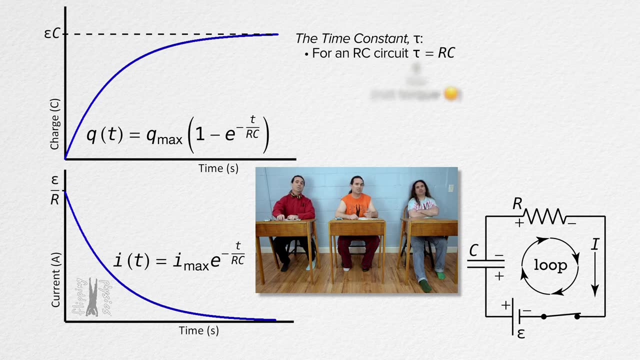 The symbol for the time constant equals resistance times, capacitance. Another construction constant is the lowercase greek letter tau. Before we discuss further what the time constant actually is, Bobby, please determine the units for the time constant of an RC circuit. The units for the time constant of an RC circuit? Well, the time constant equals resistance times. 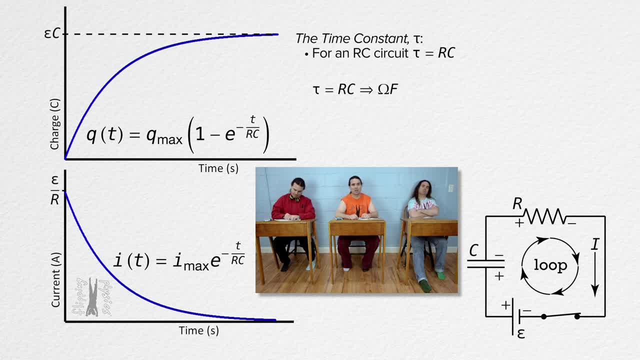 capacitance. The units for resistance are ohms and the units for capacitance are farads. Resistence equals electric potential difference over current, so ohms are volts over amps. Capacitance equals charge over electric potential difference, so farads are coulombs over. 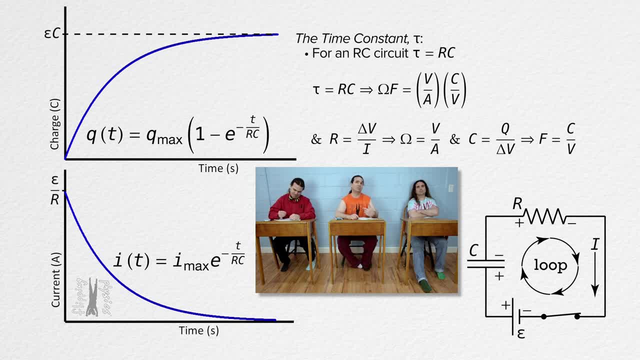 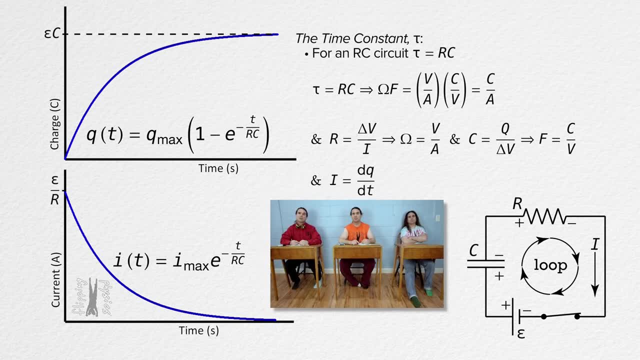 volts, Volts cancel out, and we are left with coulombs over amps. Amps are well current equals the derivative of charge with respect to time. so amps are coulombs per second, Coulombs cancel out, and 1 over 1 over 1.0V. 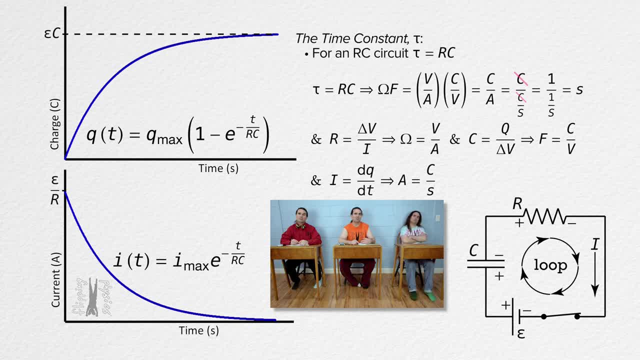 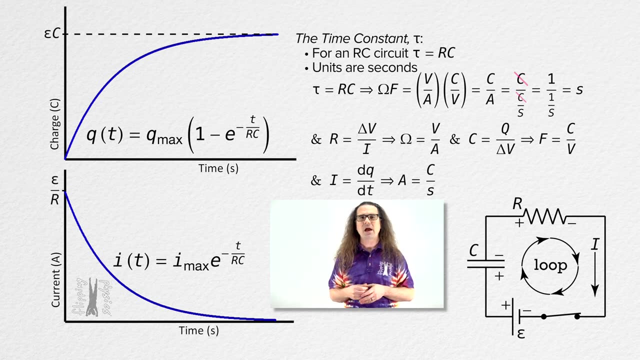 … … …. seconds is just seconds. The units for the time constant are seconds, Which makes sense. It's the time constant. Thank you, Bobby. And I agree it makes sense that the units for the time constant would be seconds, the base SI unit for time. Now, in order to understand what the time constant. 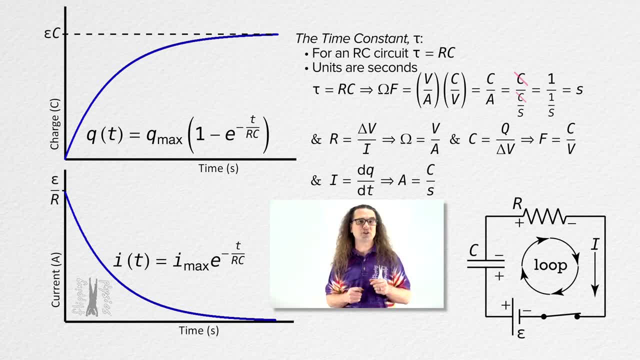 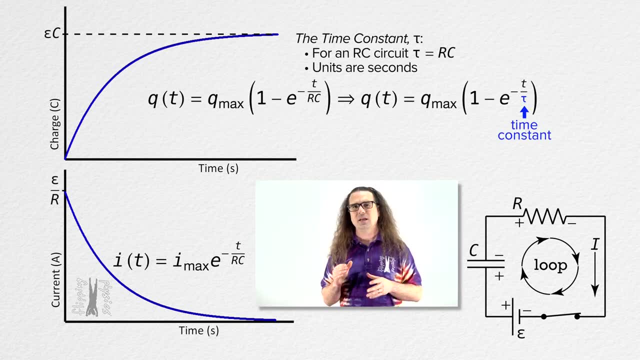 actually is. let's go back to the equation for the charge on the capacitor as a function of time And replace resistance time capacitance with the time constant. And now let's determine the charge on the capacitor after a time of one time constant after the switch has closed. All we have to do is 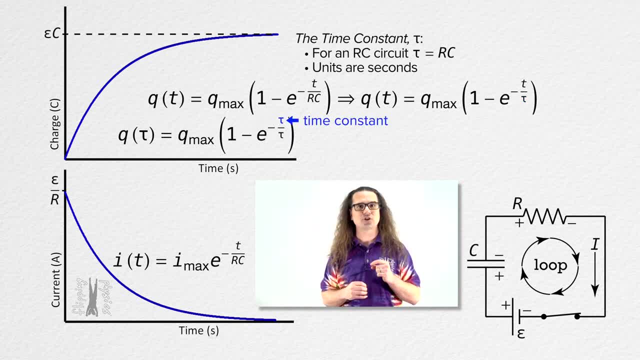 substitute one time constant in for time t in our charge equation We get e to the negative time constant over time constant, which is e to the power negative 1. Class: what does e? raised to the power negative 1 equal 0.368..